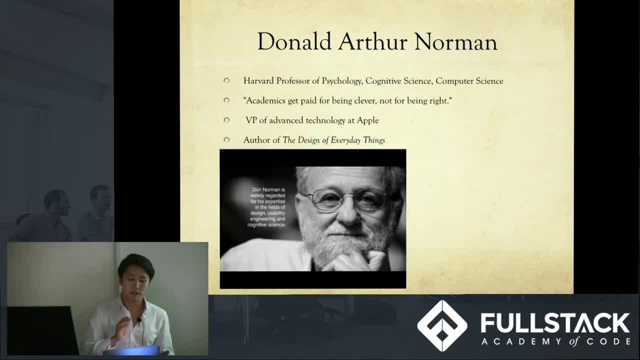 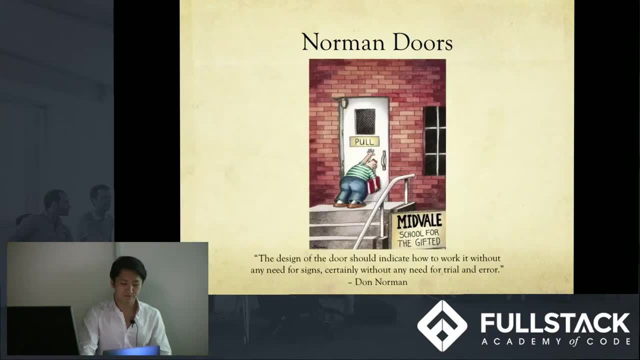 But I want to focus on mainly one concept that was coined after him due to his book The Design of Everyday Things, and it's called Norman Doors. The idea of Norman Doors captures and illustrates very well the underlying principles of UX. A Norman Door is a design where it tells you or signals you. 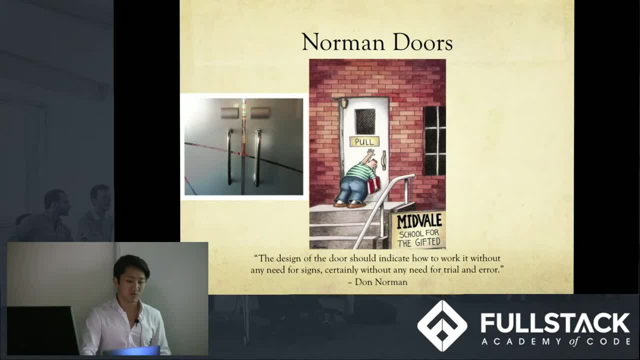 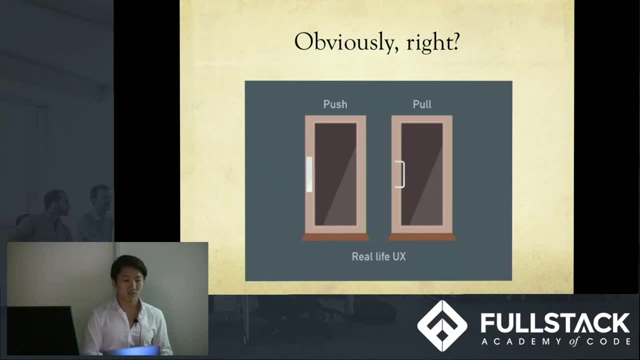 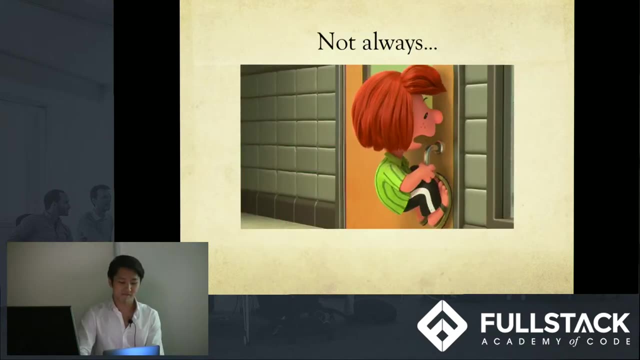 to do something that is exactly the opposite of what you're actually supposed to do and needs a sign to correct it, Whereas really good and well-made designs are so obvious that you probably never have to think about them, which isn't always the case, 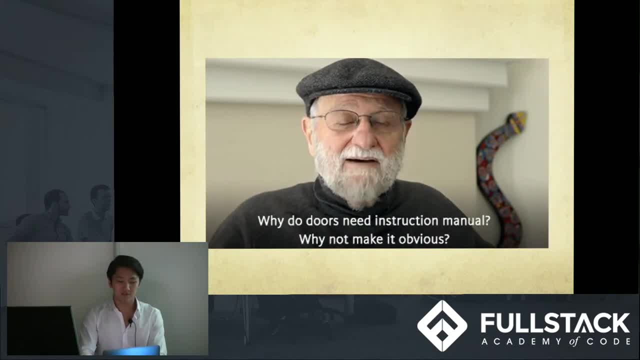 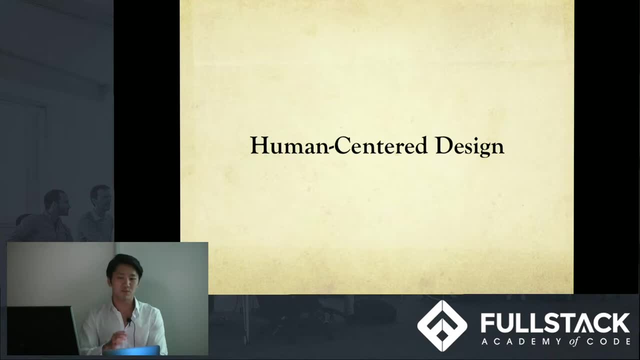 Why do doors need instruction manuals? Why not make it obvious and intuitive? And this is what he calls human-centered design, and it's divided into two major principles: Discoverability and feedback, And this forms the basis of how designers and engineers work today. 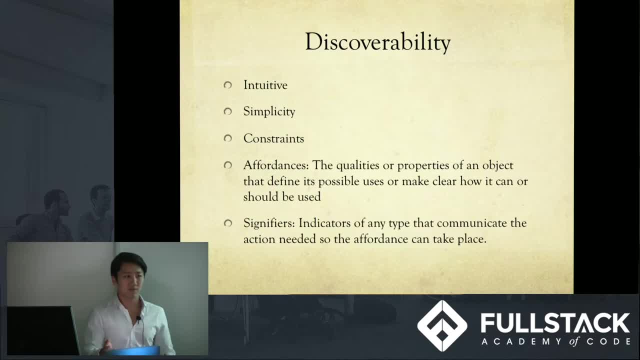 First discoverability is when you look at something, a design, an object, a product, anything. I should be able to figure out what operations I can do and which direction I should take it. In order to achieve this, we want to maintain simplicity and constraints. 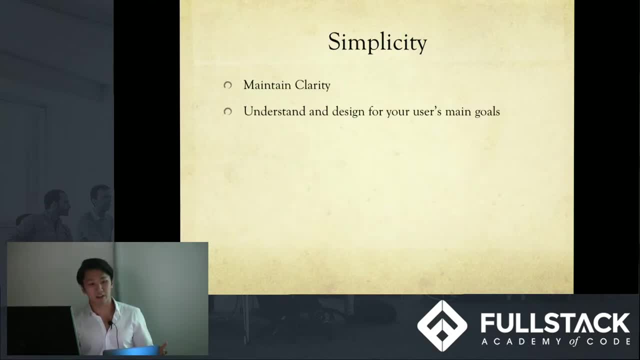 To achieve simplicity. we want to provide clarity and understand what the user really wants. Let's see some examples. So the world's most popular search engine, Google, commands over almost 70% of the world's market share, and it directs the user's attention to one thing, and one thing only. 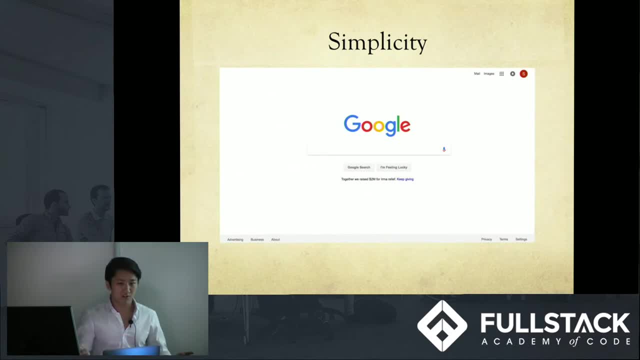 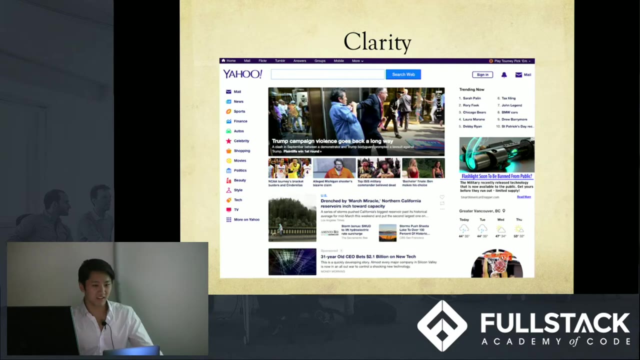 the search bar. It's void of any other noise or distractions that might take away attention from the user's main goal And, as you know, they've seen massive success by staying true to this minimalist and straightforward design. Yahoo, on the other hand, 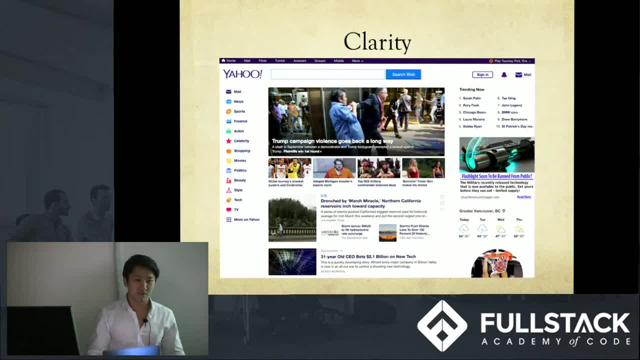 their homepage has so many things that divert your attention away from their main goal, and just having too many things going on at once. Maintain clarity by designing for your user's main goal and don't confuse your users with extra information that's irrelevant to achieving their main goals. 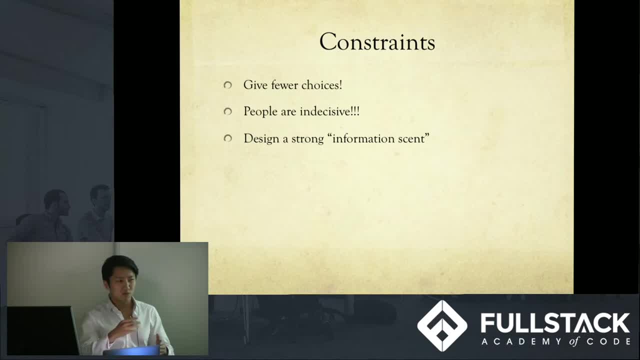 Now. constraints are good because it helps you determine a course of action by limiting the amount of possible actions. People are generally indecisive in today's age, so it helps remove the indecision and confusion as well. The best UIs will guide users with clear steps. 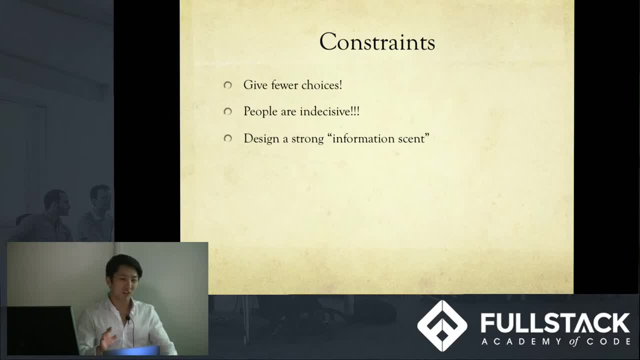 to arrive at their desired destination, and this is called leaving a strong information scent. So when it comes to dating, it's probably a good thing to have a lot of options, but when it comes to this, too many options can make people sad. 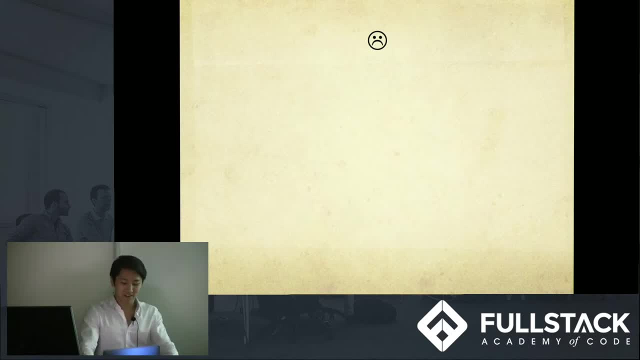 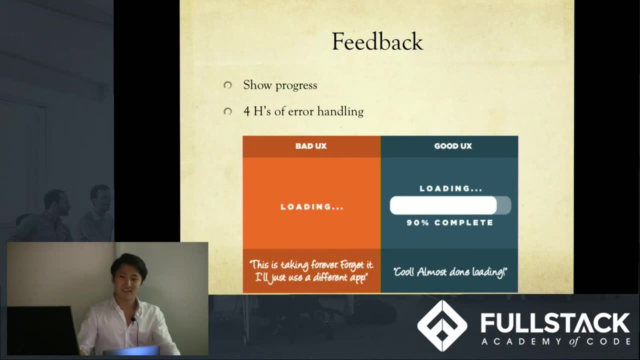 And here's an example of what might break mine and your heart. Yeah, Feedback. It's about providing information to the user about what has taken place and what your progress is to your goal. Even something simple as this loading bar lets users feel a little happy. 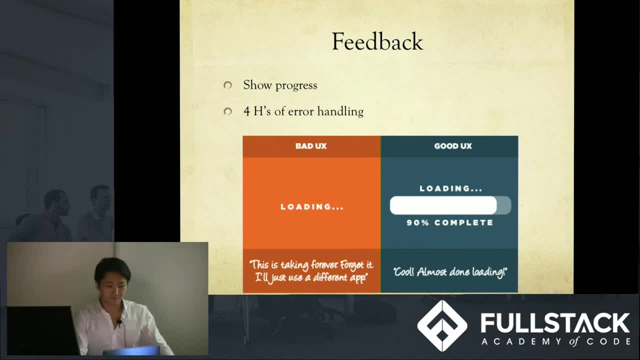 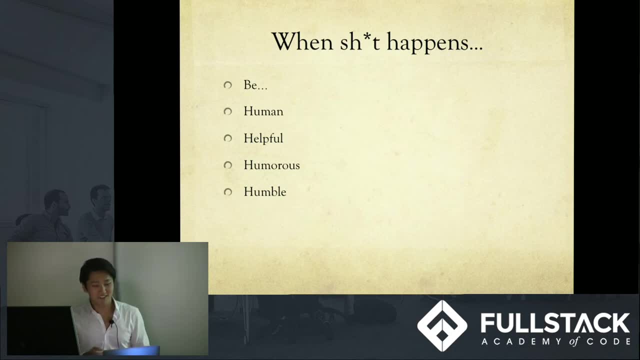 by knowing how close they are to their goal. And sometimes they're unavoidable, but they happen. They're errors And when they do happen, error messages should be human, as in it should feel like you're talking to a person and not a robot. 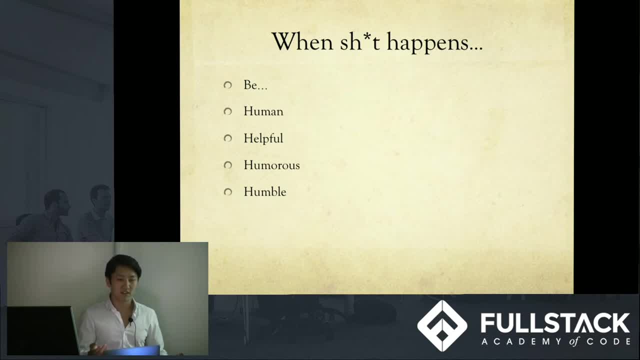 It should be helpful. It should provide some next steps that you can take. Humorous: There might be some agitation, so if you can ease that tension, then that's good And humble. Don't blame the user, even if it might be their fault. 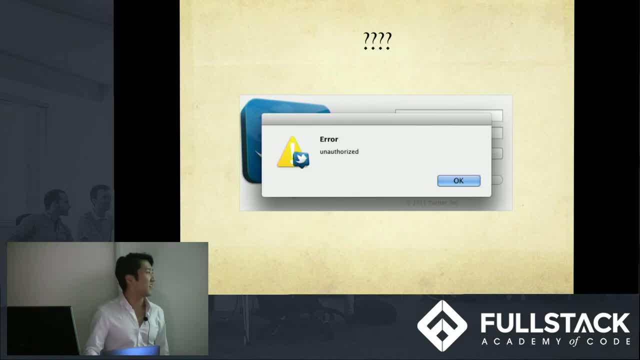 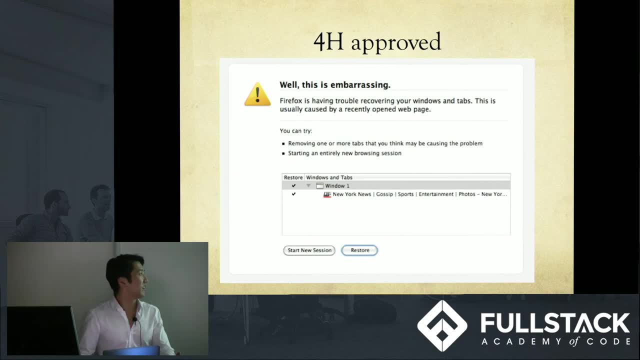 Bad example. What is this? I'm not sure, And this is what I give a 4H certification. So web browser crash from Firefox. Well, this is embarrassing. That's human and it's a little humorous. Firefox is having trouble. 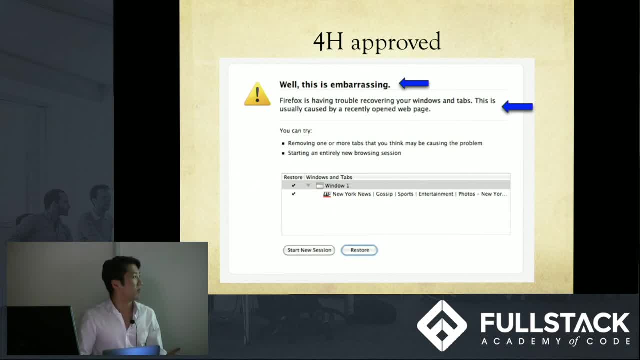 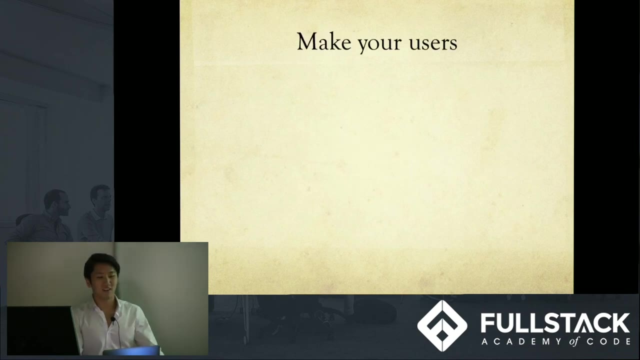 recovering your windows and tabs. This is humble- It's not blaming the user- And helpful. You can try removing one or more tabs, or you can start an entirely new browsing session. So, finally, make your users happy by following these principles. That is all, Thank you.